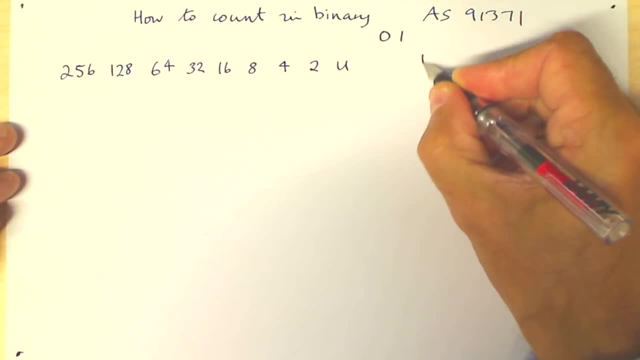 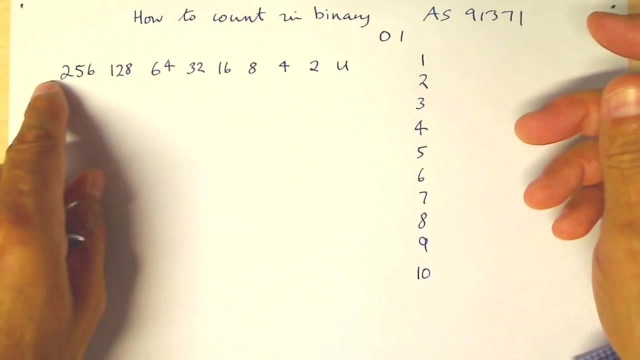 to show you how numbers work over here. So we're going to do a decimal number. It's going down the side. I'm going to count to 10 to start with. So to do the number 1 in binary, we go along here. 256 is too big, 2 is too big, So we 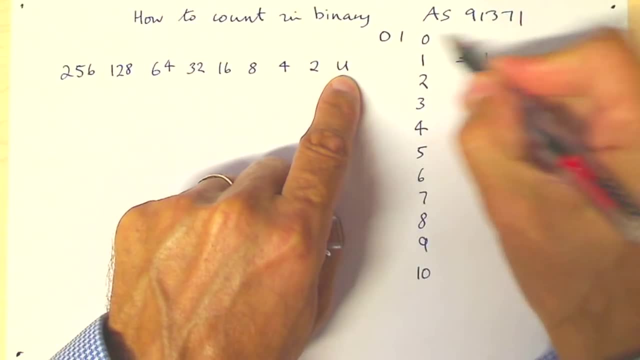 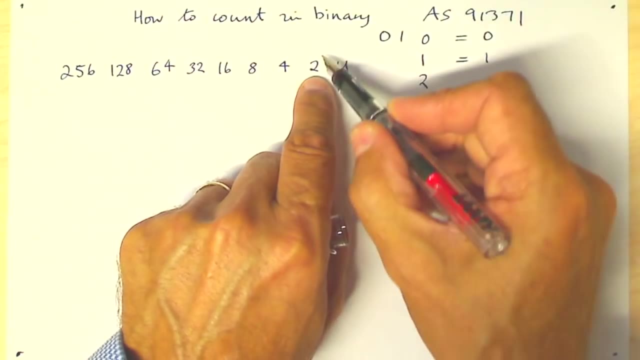 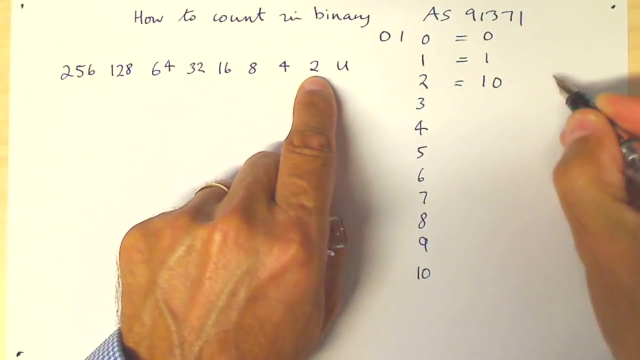 just have 1 unit. So 1 equals 1.. Of course, 0 equals 0. So we're going to do a number 2.. So go along. We get to number 2 here. So we would have 1, 2 plus no units. So this: 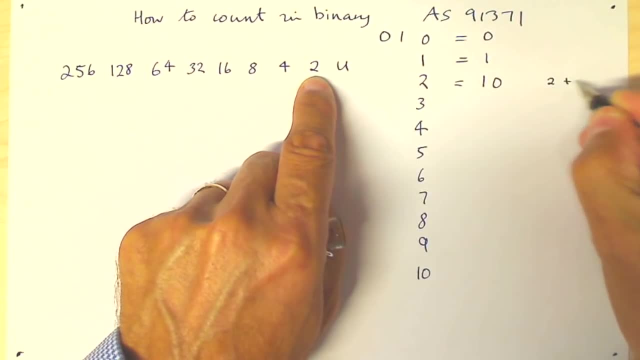 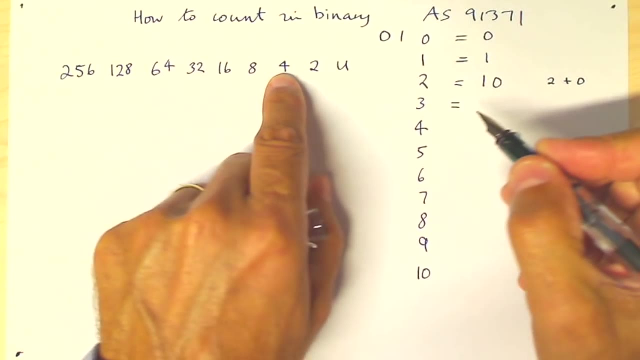 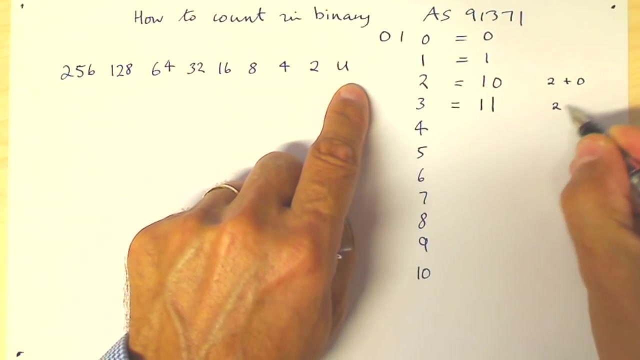 how it's worked out. It's a 2 plus 0.. So we've got a 2 plus 0.. Number 3, work along. Now 4 is too big, So we'd go we need a 2 and a 1.. So how is that worked out? It's a 2 plus. 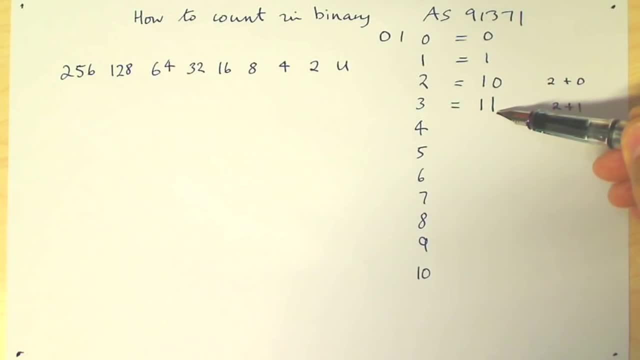 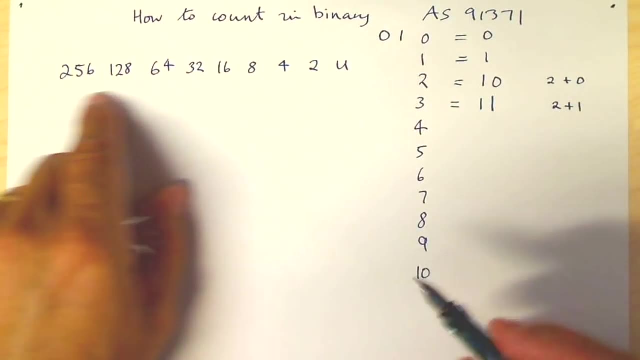 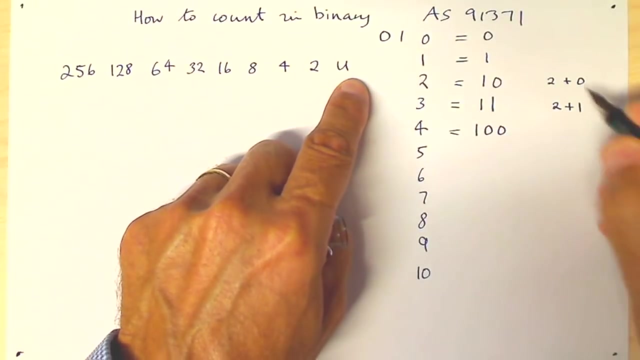 a 1.. Notice that we don't call it 11.. OK, 3 is represented by the two digits 1 and 1.. So let's do 4.. We need a 4.. No 2s, no units. How it's calculated, It's 4 plus 0 plus 0.. 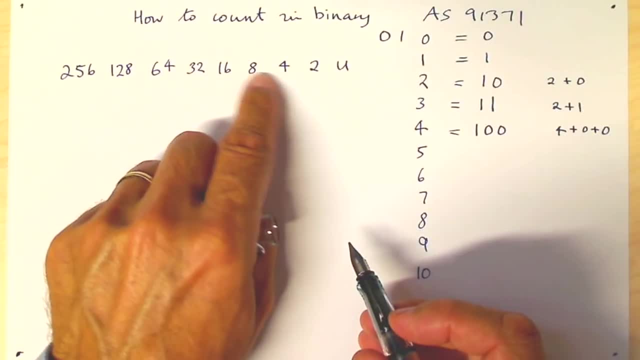 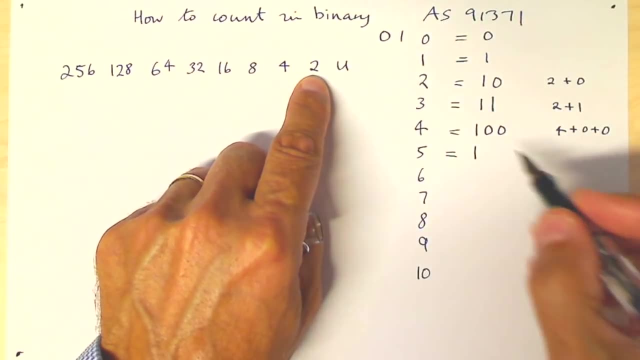 Let's do 5.. An 8 is too much, So to make up a 5, we will need a 4.. Now, 4 and 2 is 6, so that's too much. So we don't need a 2 and we need a unit. So how it's worked. 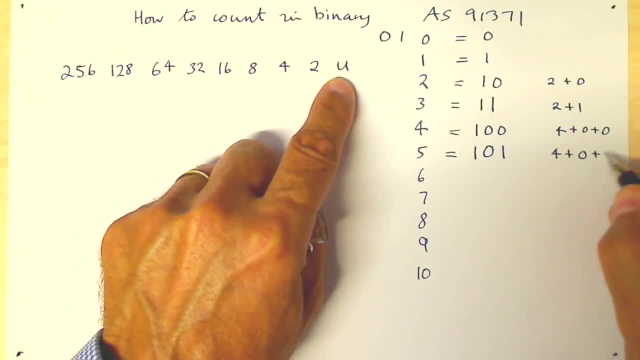 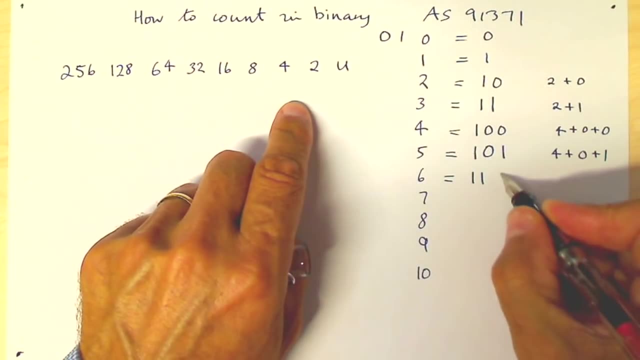 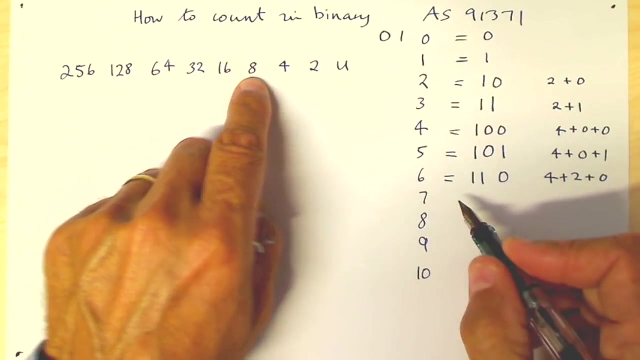 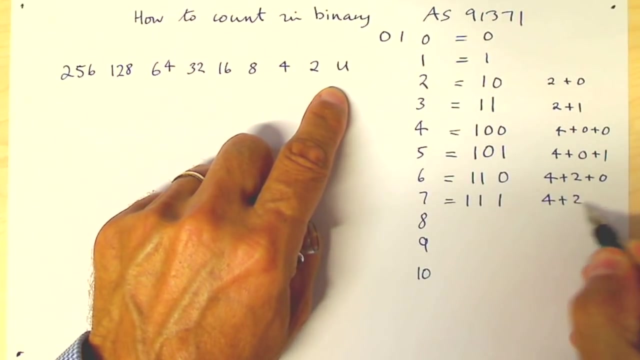 out is 4 plus 0 plus 1.. So 6 is a 4 and a 2 and no units. And it's dead easy. So we can do 7.. 8 is too big, So we do a 4, a 2 and a 1. And we go into 8. So we've got an. 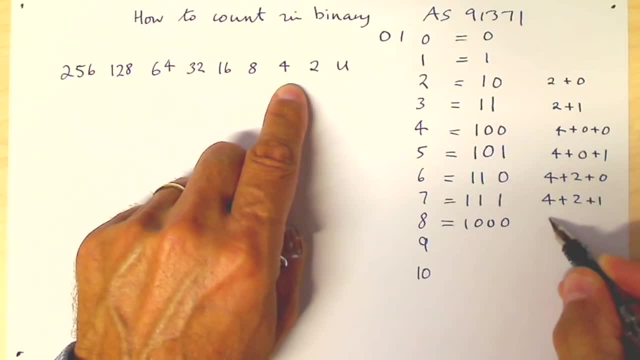 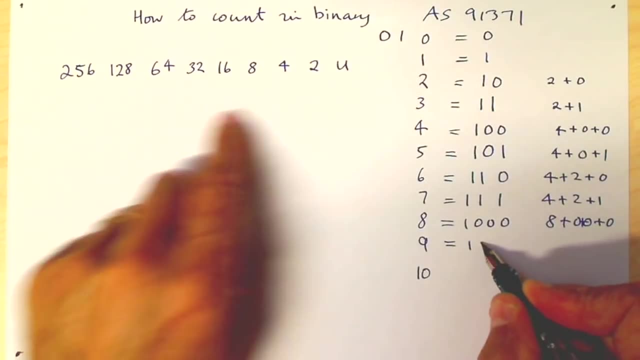 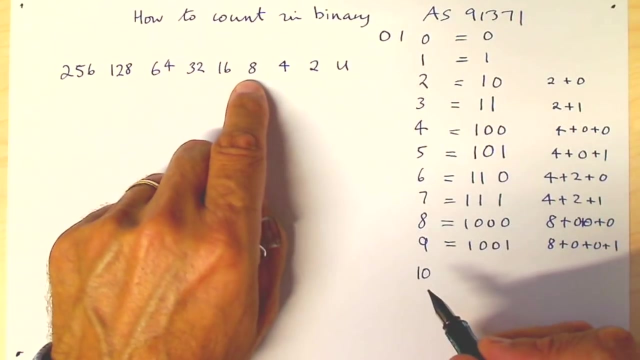 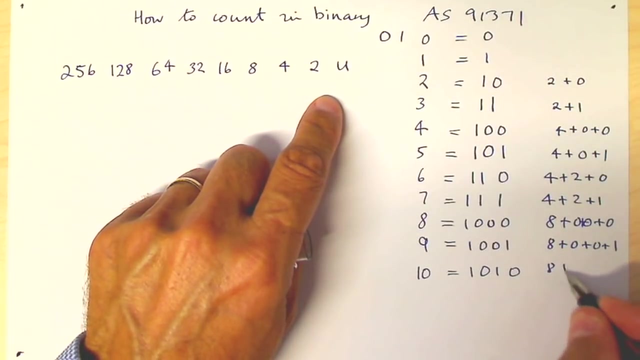 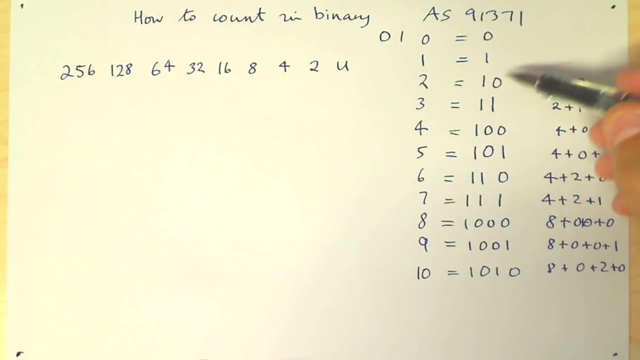 8. No 4s, No 2s, No units. 9 will be an 8 and a 1. And a 10 will be an 8 and a 2.. OK, there's an interesting pattern. We can see that. 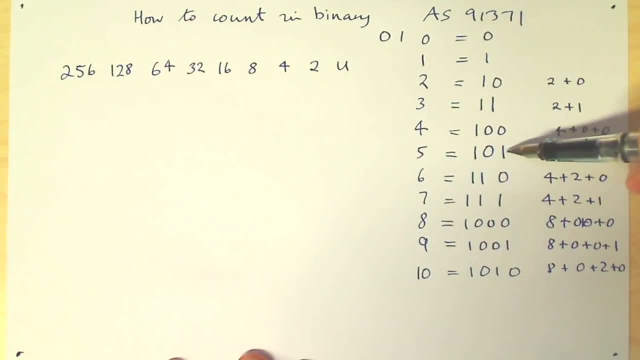 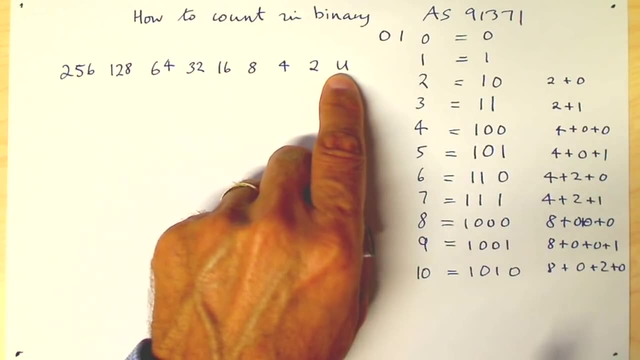 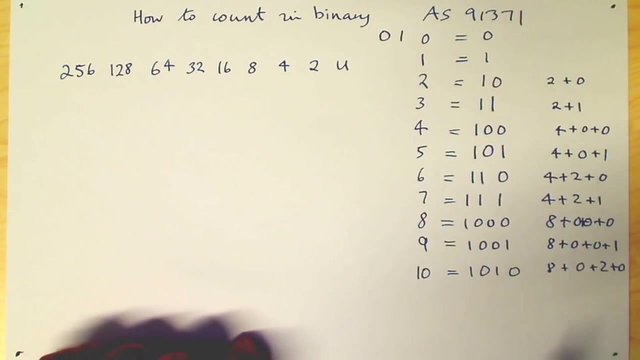 odd numbers always have a 1 as the last digit. That's kind of obvious really, though, because an odd number must have a single digit at the end, because all the rest aren't even. OK, we'll just do a slightly more complicated one. I'll do. 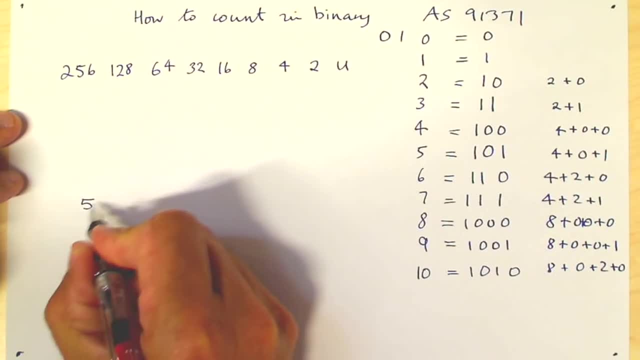 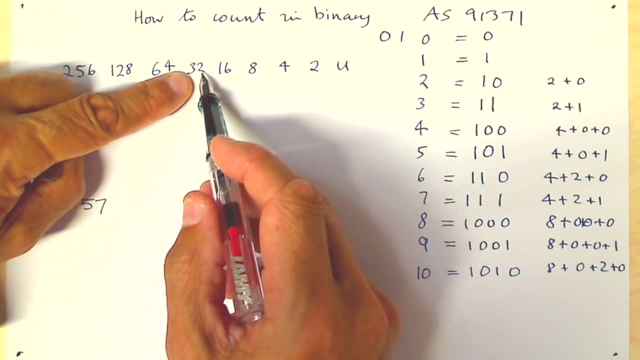 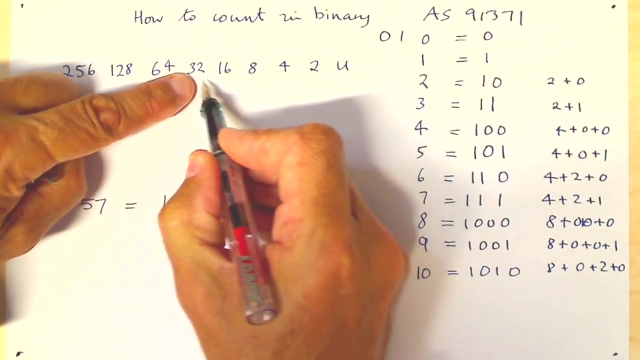 number 57. So to calculate 57, we do this, We go along and we basically say: OK, which number is the largest number that comes in there? So we've got 32.. So 32.. Now 32, work along 32 and 16 is 48. We're looking. 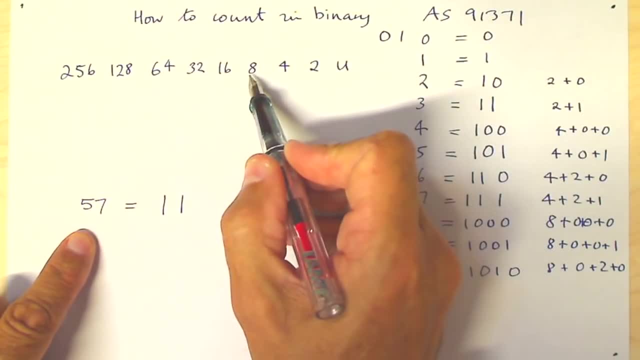 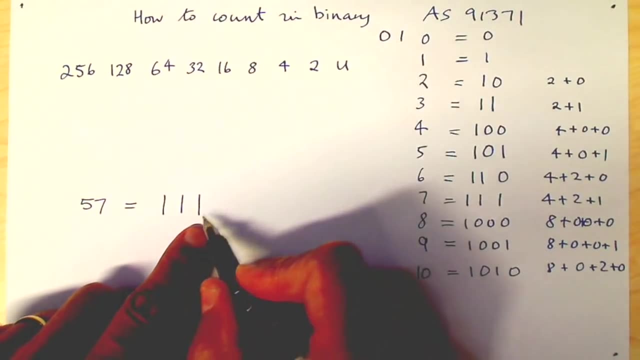 for 57.. So we've got a 48.. 48 and 8 is 56.. So we want one more. So we've got 48, and 8 is 56. So we don't need a 4.. We don't need a 2.. 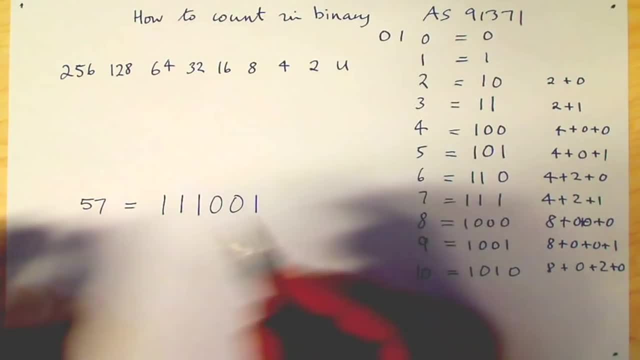 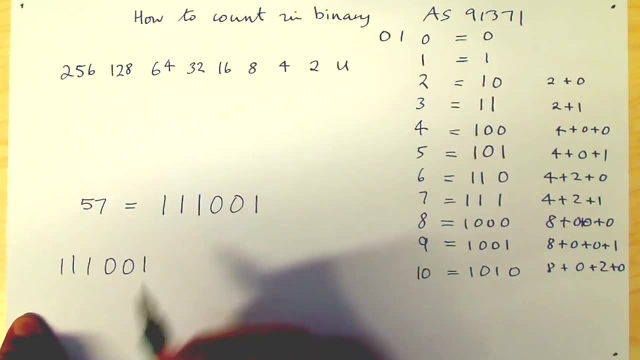 We need a 1.. So that should be 57.. Let's double-check it, So we've got one, one, one, zero, zero one. So we go units twos, fours, eights, sixteens and thirty-twos So. 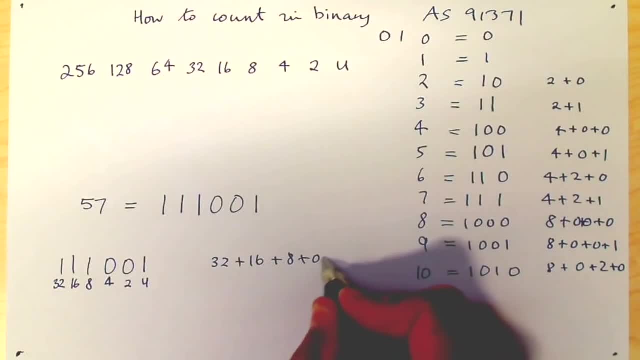 we've got 32, plus 16, plus 8, plus 0, plus 0, plus 1.. What else do we have? Well, again we've got theironomian units, So you can get an Motor. We keep the process. http//attached现在. 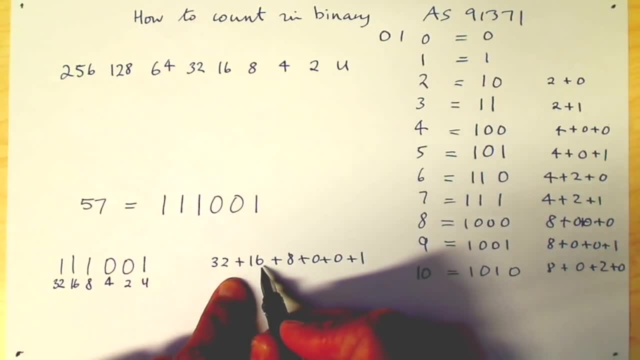 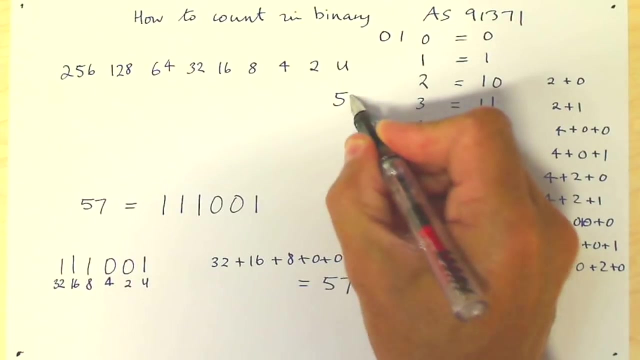 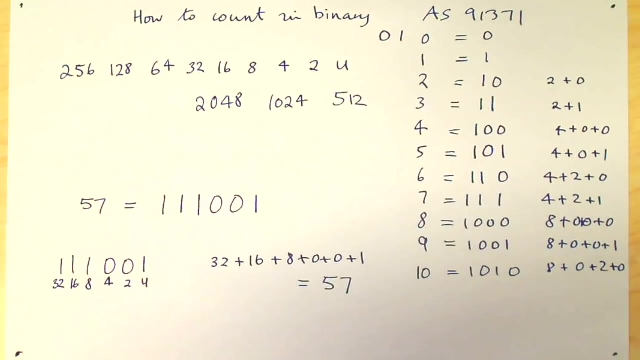 1,, 32, and 16,, 42,, 48,, 56,, 57. That works for any number. If we were to quickly calculate what numbers go beyond 2,, 5,, 6,, they're really easy: 5, 1, 2,, 1,024,, 2,048, and so on. 4,096.